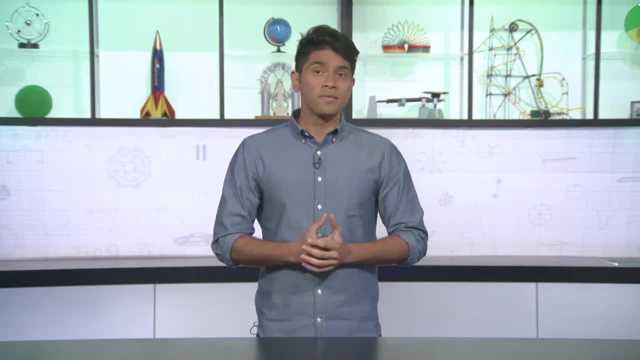 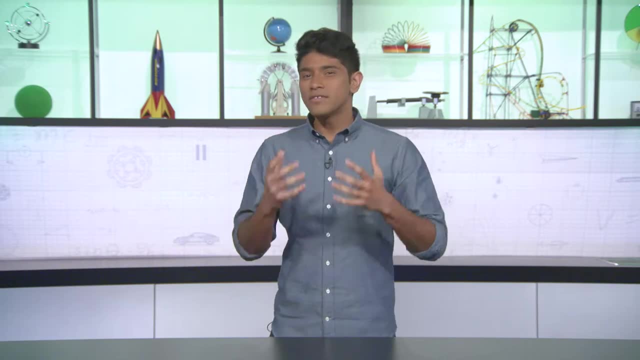 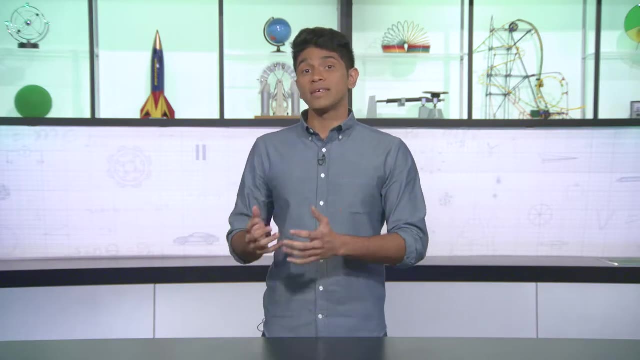 of energy, electric potential. energy is a scalar quantity But unlike other scalar quantities like speed and temperature, it can be positive or negative. Now, it has nothing to do with direction, like it would in a vector quantity, but is determined by whether energy is lost or gained. 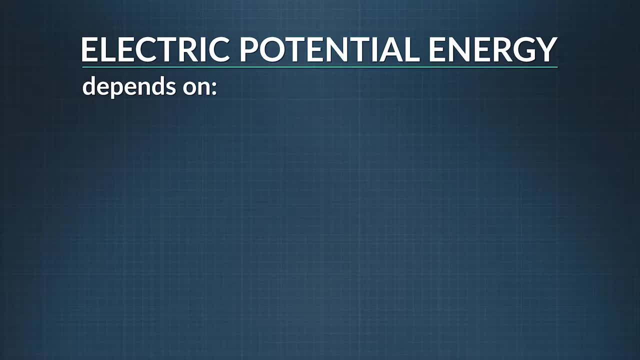 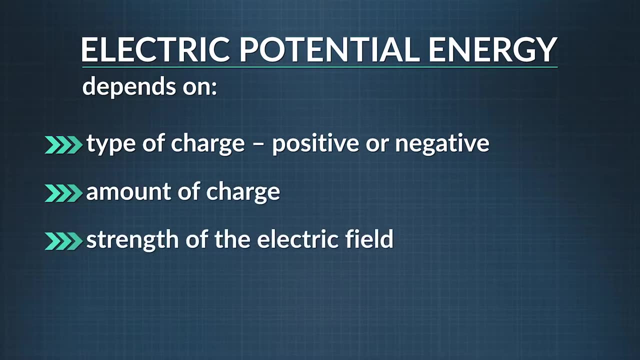 in a system, Electric potential energy depends on three things: The type of charge, whether it's positive or negative- the amount of charge and the strength of the electric field it's in. Electric potential energy uses the same units as gravitational potential energy joules. We can. 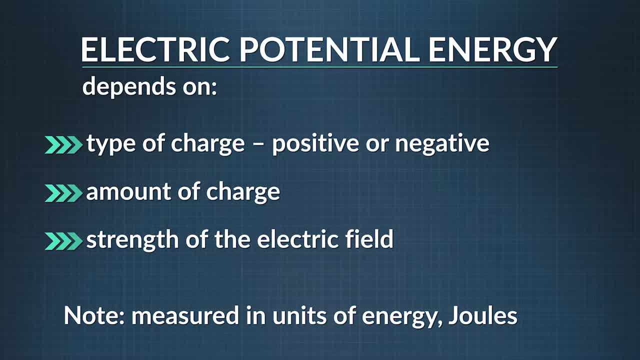 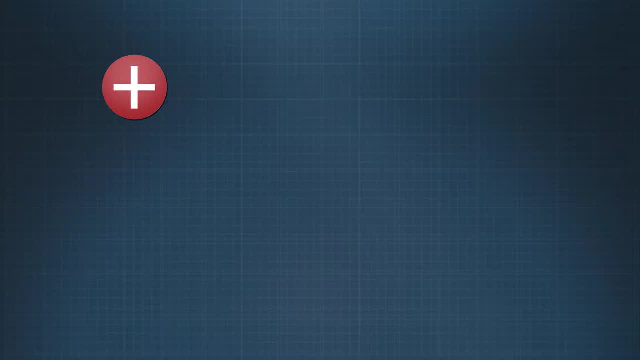 figure out how much energy a system has by considering the electric charges and fields that are involved. Let's do a quick calculation to see how that works. Say you have a charge of positive 5 times 10 to the negative 12 coulombs creating an electric field. If a second point, 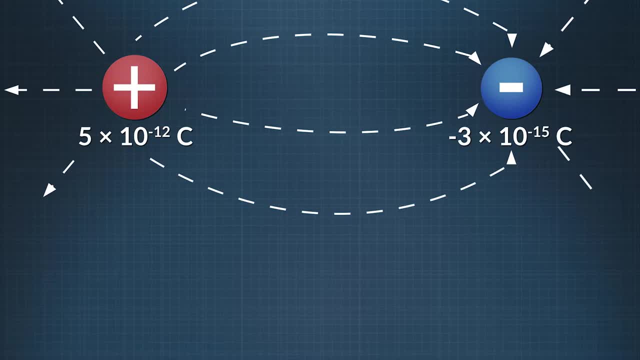 charge of negative 3 times 10 to the negative 15 coulombs is 7 meters away. what is the electric potential energy stored by the second charge? Electric potential energy equals the constant k times the product of the charges divided by the distance between them. Now we plug. 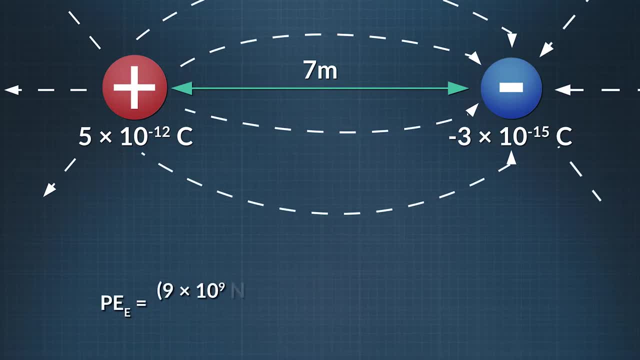 in what we know, k is 9 times 10 to the ninth Newton meter squared per coulomb squared. This is multiplied by the first charge, positive 5 times 10 to the negative 12 coulombs, times the second charge, which is negative 3 times 10 to the negative 15 coulombs. If a second charge is 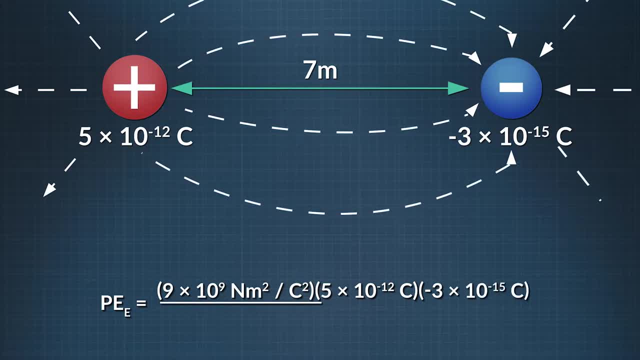 negative 5 times 10 to the negative 15 coulombs. the second charge is 10 to the negative 15 coulombs divided by a distance of seven meters. Plugging these values into the electric potential energy equation gives us negative 1.9 times 10 to the negative 17 Newton meters. Since a 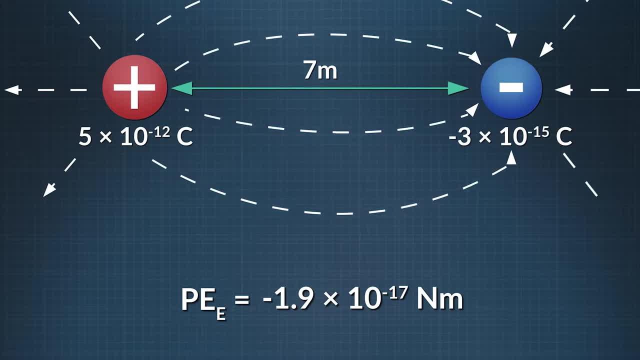 Newton meter equals 1 joule, our answer is that the electric potential energy of the second point charge equals negative 1.9 times 10 to the negative 17 joules. Notice that the sine of each charge matters and the answer is a negative number. the negative sign tells us that 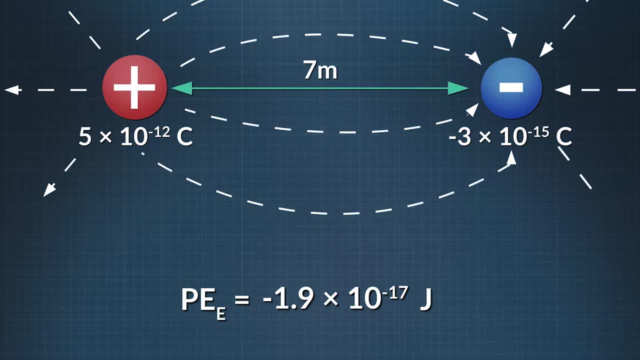 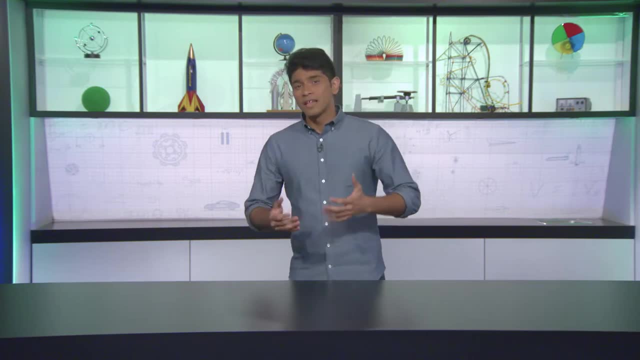 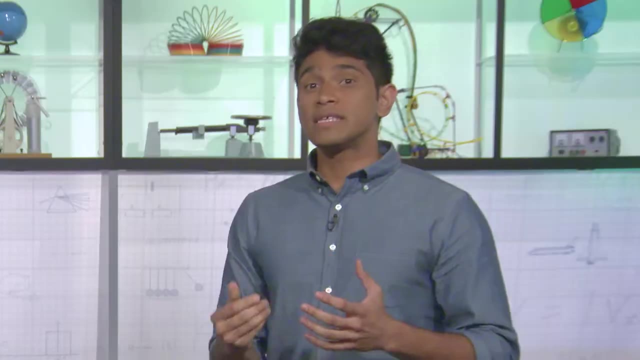 work must be done on the system to keep these charges apart. so electric potential, energy is the ability of a charge to do work. but how does that? well work. let's see. we have two charged plates. the top plate is positively charged and the bottom plate is negatively charged. you can see the 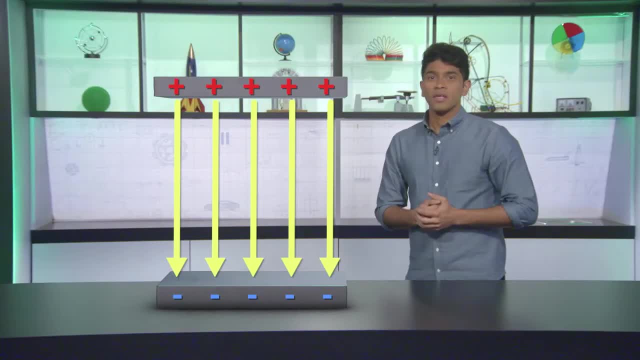 electric field lines going from the positive plate to the negative plate. let's put a positive charge in the electric field. work must be done to push a positive charge towards the positive plate or away from the negative plate when the positive charge is moving opposite the direction of the. 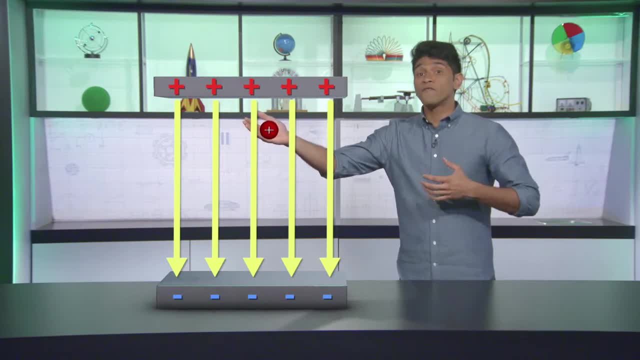 electric field. we call that moving up the field. the further up the field the positive charge goes, the more work you have to do, like if you were pushing a ball uphill. when the positive charge is here near the positive plate, what kind of electric potential energy does it possess? 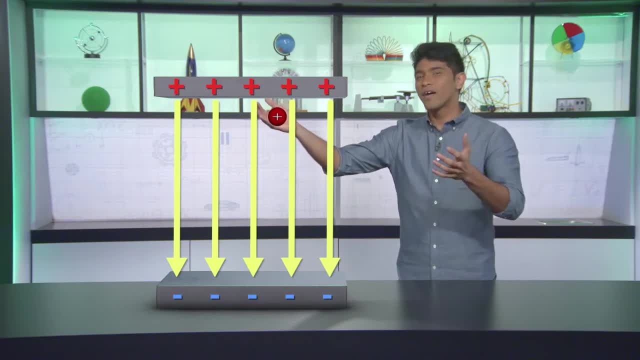 if you said it's high or strong, That's right. In fact, we can say that the charge has maximum electric potential energy. The charge doesn't want to be up here, So if you let it start to move, it will be repelled. 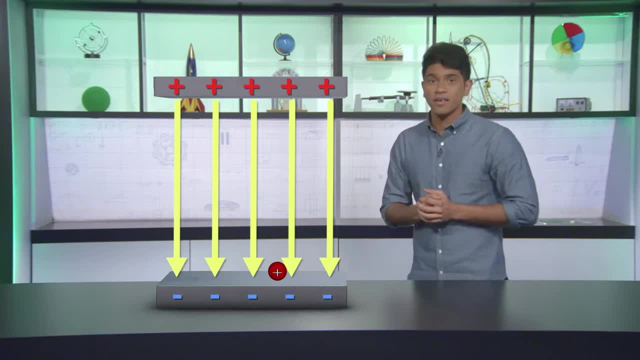 away from the positive plate and, attracted towards the negative plate, It will accelerate all the way down While it's falling. what's happening? Think back to gravitational potential energy of the dam, because this works in a very similar way. If your answer was that, 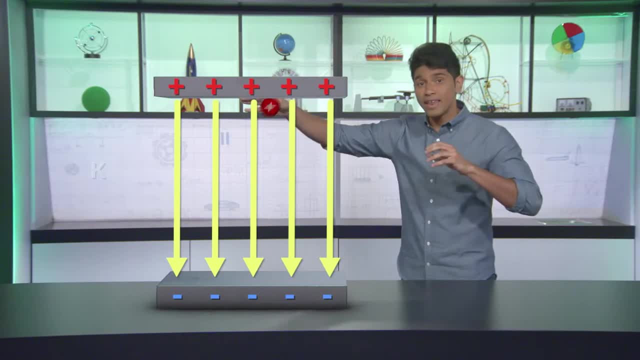 the electric potential energy is decreasing. being converted into kinetic energy, you're right. When it reaches the negative plate at maximum velocity, how much electric potential energy is left? If you said none, you got it right again. It has no electric potential. 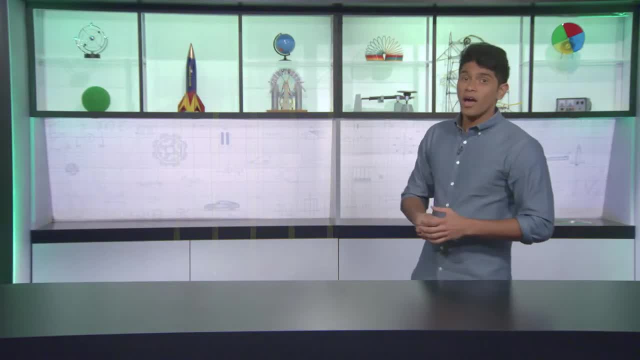 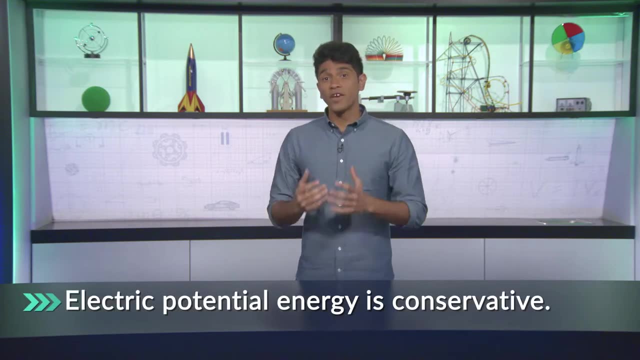 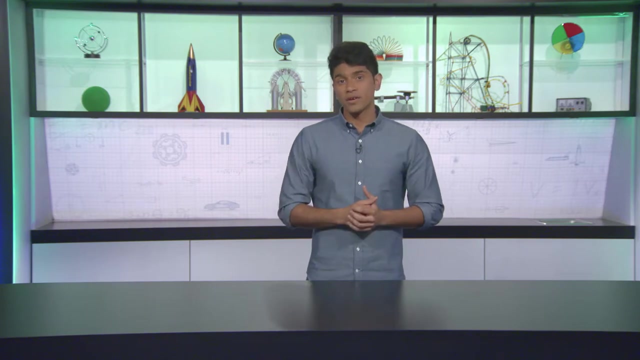 energy left, It all changed to kinetic energy. Another important characteristic of electric potential energy is that it is conservative, which means that it obeys the law of conservation of energy. Whatever an object loses in the potential energy, it gains in kinetic energy, and vice versa. 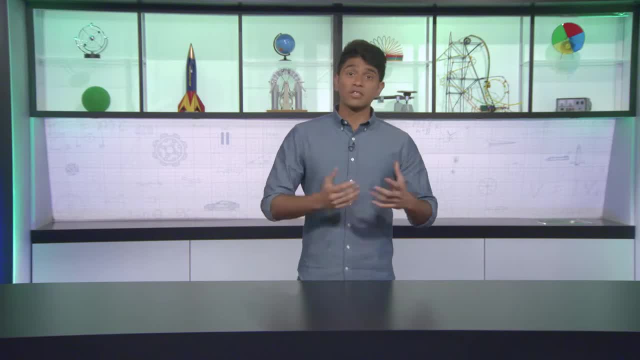 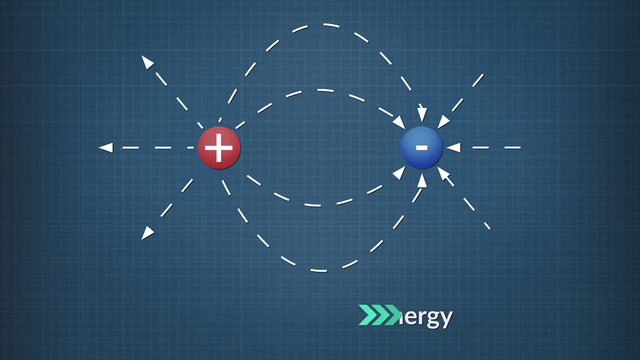 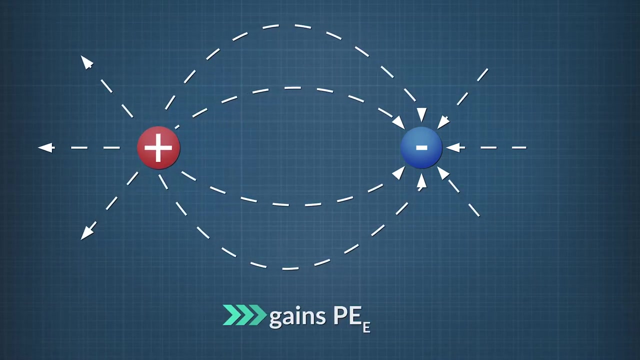 Now let's look at what happens to electric potential energy in different scenarios. A positive charge near another positive charge has high potential energy. A positive charge near a negative charge has low potential energy. A positive charge gains electric potential energy when it is moved in a direction opposite the electric field. A negative charge gains. 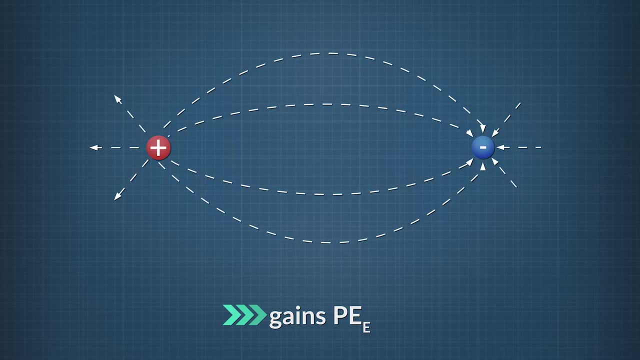 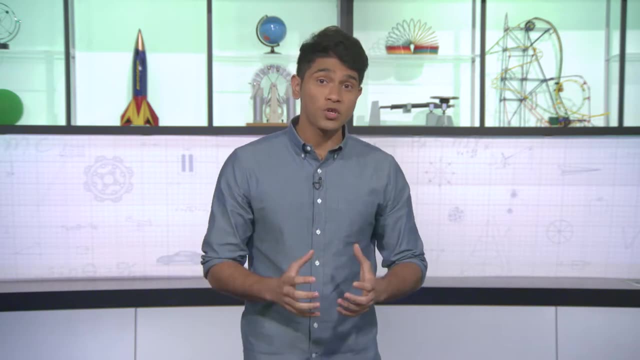 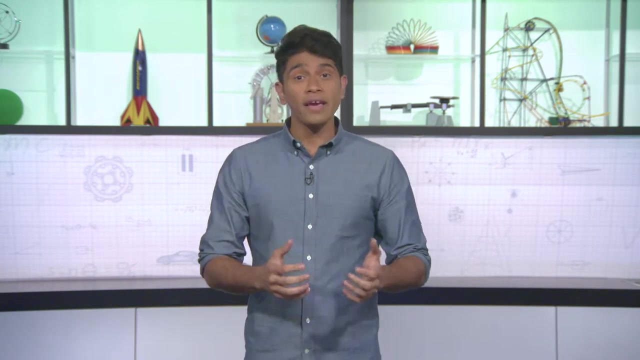 electric potential energy when it is moved in the same direction. Those are the basics of electric potential energy, which has a strong resemblance to gravitational potential energy. Both depend on the position of an object in a field and both can be positive or negative. To understand the equation for electric potential energy, 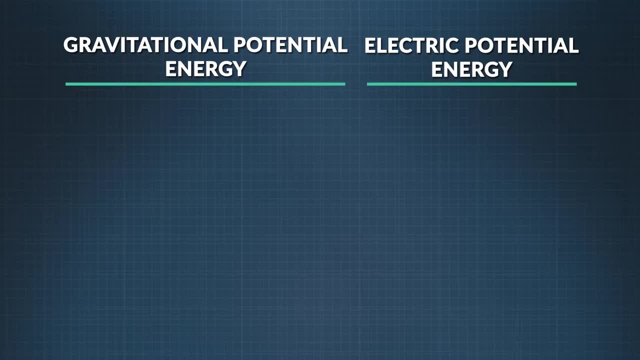 stored by a charge between two charged plates. let's look at the equation for gravitational potential energy and compare it to electric potential energy. The potential energy of an object due to gravity equals its mass times gravitational field strength times its height. So the electrical equivalent of mass is charge, which is q, Where g represents. 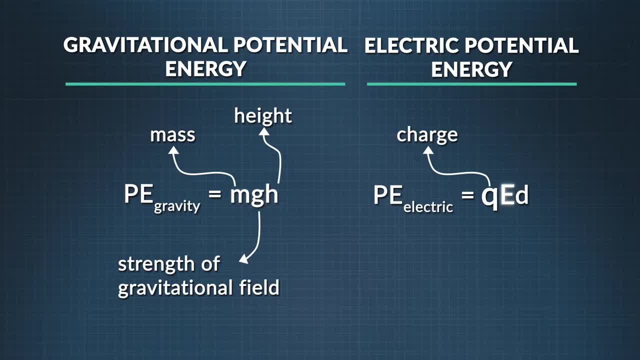 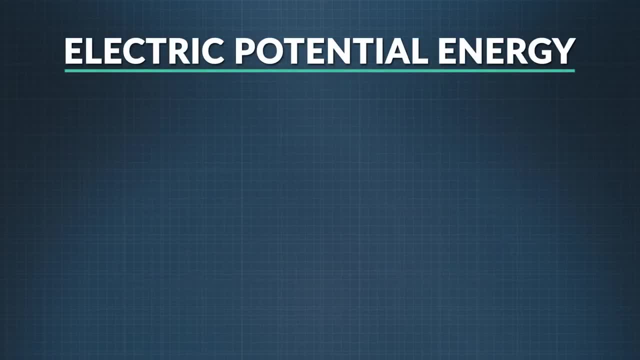 the strength of the gravitational field. we replace it with electric field e, And the height above ground becomes the distance above the bottom plate. So we can write the equation for electric potential, energy stored by a charge between two charged plates. I'm going. 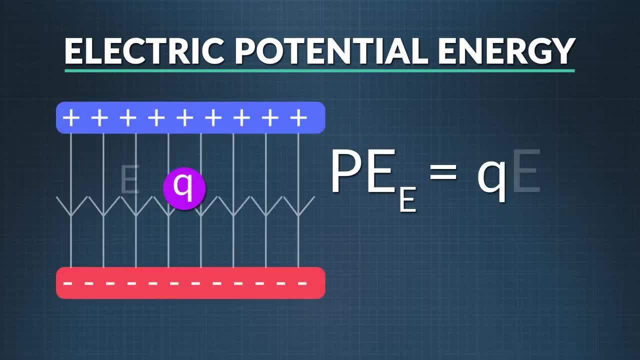 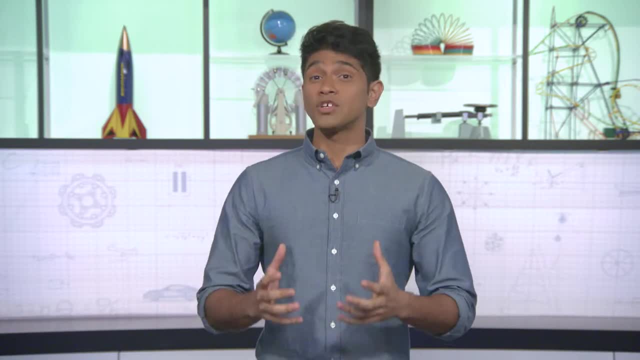 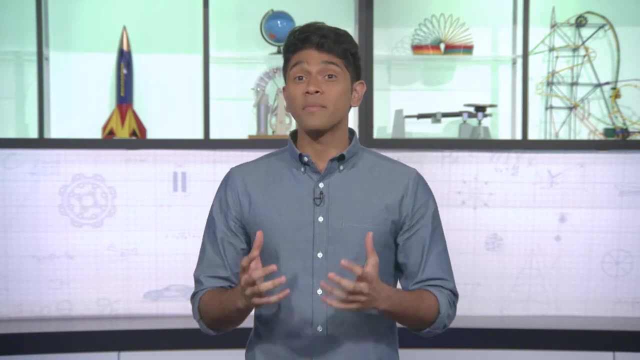 as the charge Q times the electric field, E times the distance the charge has moved within the field D, We've seen what electric potential energy is and that it is equal to the work a charge in a field can do. But how can we talk about it in a way that makes it useful to us? 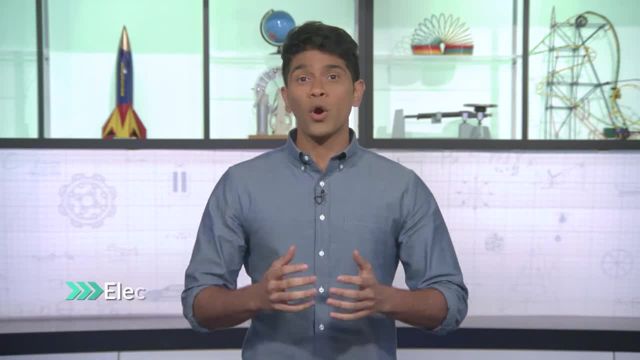 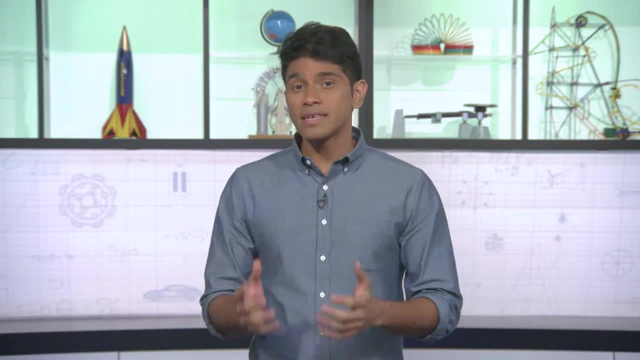 One way to describe it is per unit charge, which we call electric potential. Be careful not to confuse the two. I know the names are similar, but when we have a system with many charges, electric potential energy tells us the energy of all the charges. 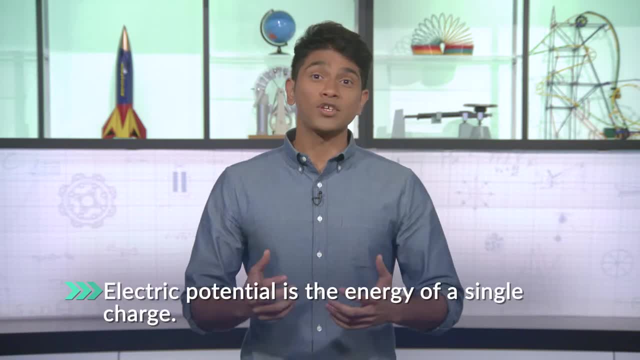 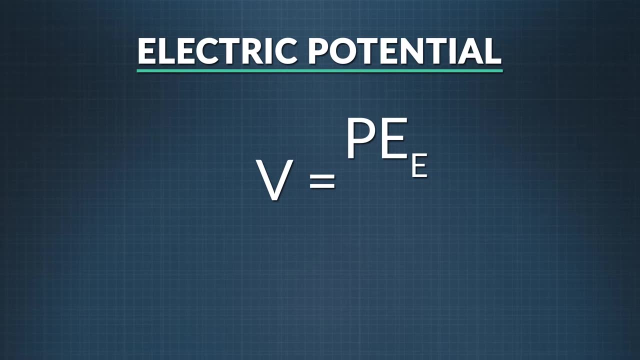 we're working with. Electric potential tells us the energy of a single unit of charge. Electric potential, represented by a V, is the electric potential energy per unit charge. Let's talk about units and that will make the difference between electric potential energy and electric potential. 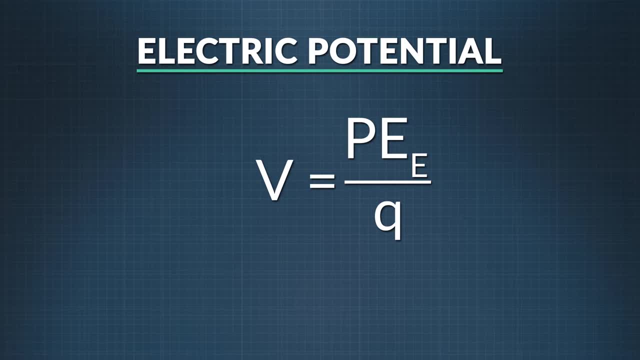 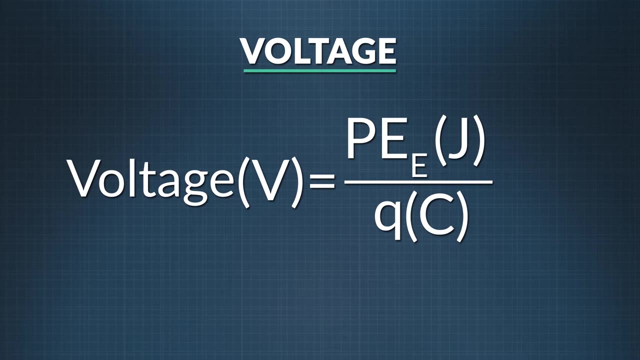 Easier to understand. Energy is measured in units of joules right. A volt is defined as a joule per coulomb. When we calculate electric potential, we can simplify the units to volts. Electric potential is also called voltage. This term connects electric potential to the electricity we harness every day. 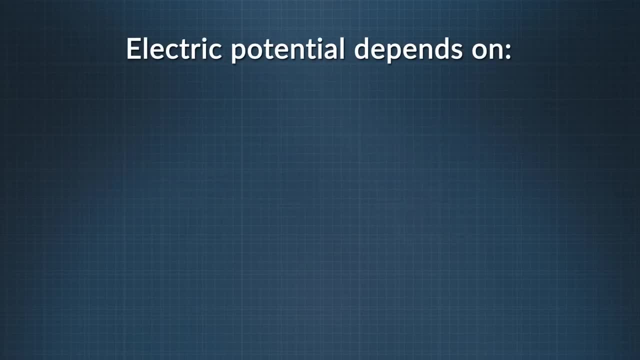 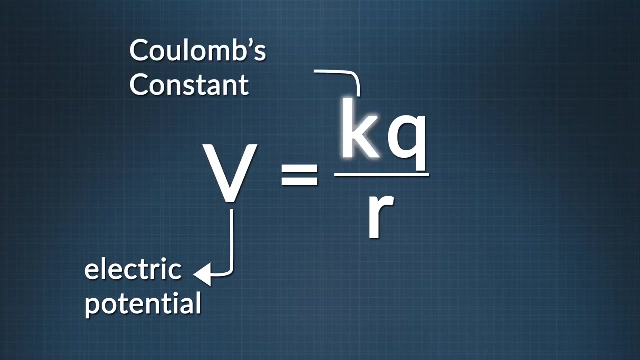 Electric potential at a point in space depends on two main factors: The amount of charge creating the potential And the distance from that charge. We can write this out as another type of equation that looks like this: Electric potential V equals coulomb's constant k times the charge responsible for the potential. 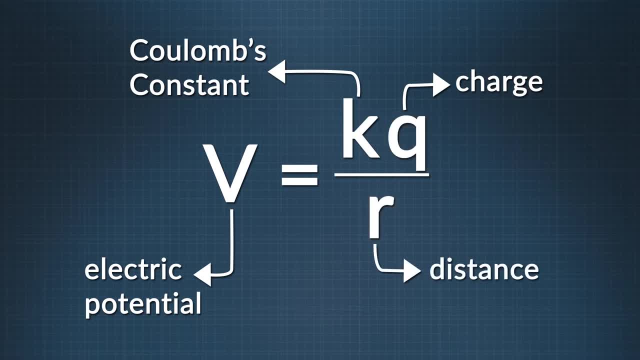 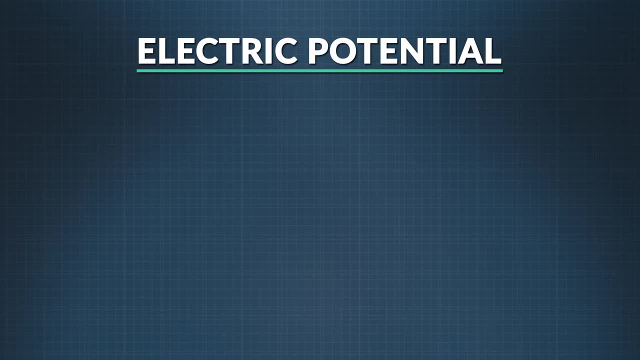 q divided by the distance r from q. What if we want to solve for electric potential at a point at which potential is created by more than one charge? The electric potential of multiple charges equals the sum of the potential V times. 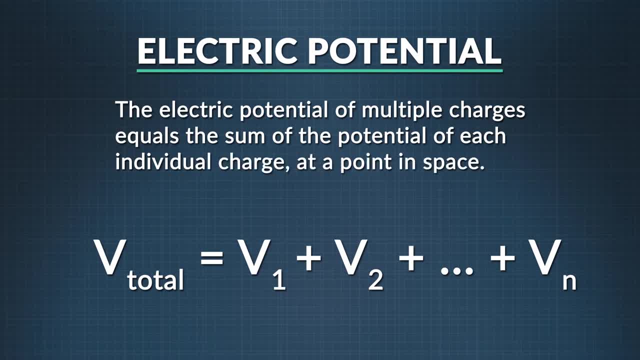 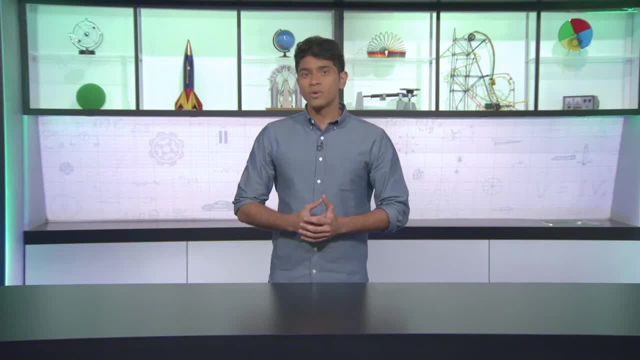 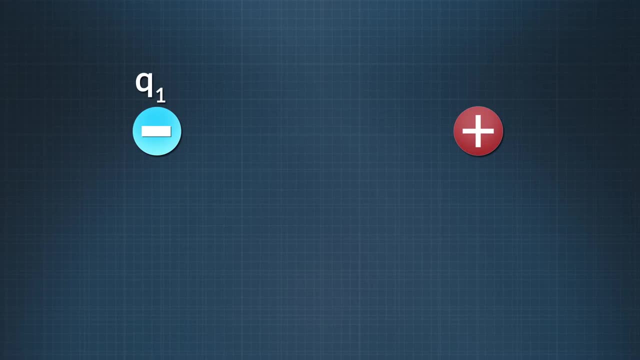 the charge. This is the potential of each individual charge at a point in space. Like electric potential, energy electric potential is a scalar quantity, so it's easy to add together. Now how does that work? Say we have two charges- q sub one and q sub two- and a point in space. we'll call point. 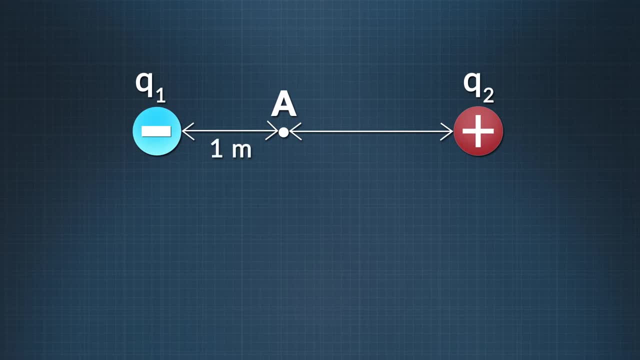 A. q sub one is one meter from point A and q sub two is three meters from point A. q sub one's charge is negative. The charge is negative five times ten to the negative six coulombs. And q sub two's is positive five times ten to the negative six coulombs. 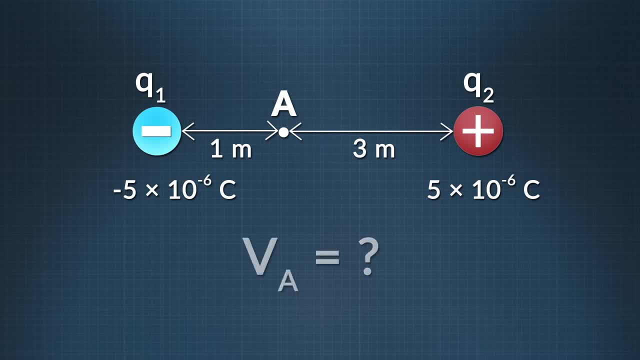 We want to know what is the electric potential at point A. Recall that electric potential V equals k times q divided by r. The potential at point A from q sub one equals k times q sub one divided by the distance between q sub one and point A. 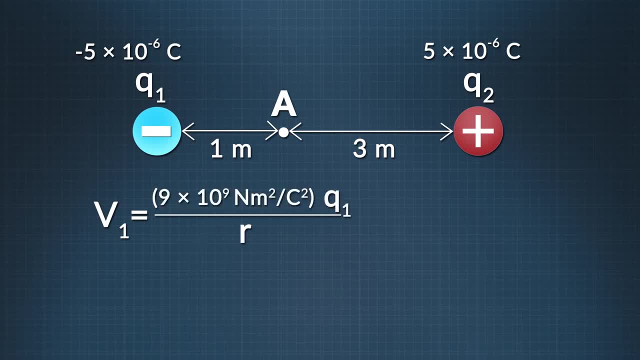 k equals nine times ten to the ninth newton meters squared per coulomb squared. q sub one equals negative five times ten to the negative sixth coulombs And r equals one meter. Plugging these numbers into the equation, we find that the potential at point A due. 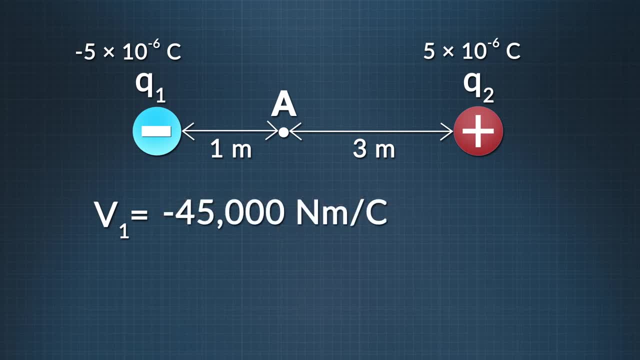 to q sub one equals negative forty-five thousand newton meters per coulomb or volts. There's still one more thing that affects the potential at point A. The potential at point A is negative forty-five thousand newton meters per coulomb or volts.